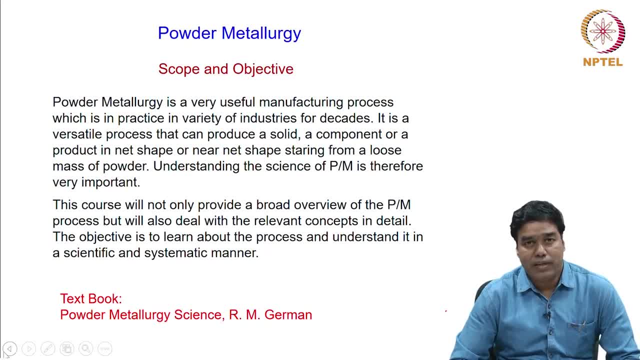 syllabus of this particular course. Powder metallurgy is a very useful manufacturing process which is in practice in variety of industries for a long time. It is a versatile process that can produce a solid, a component or a product in net shape or near net shape. 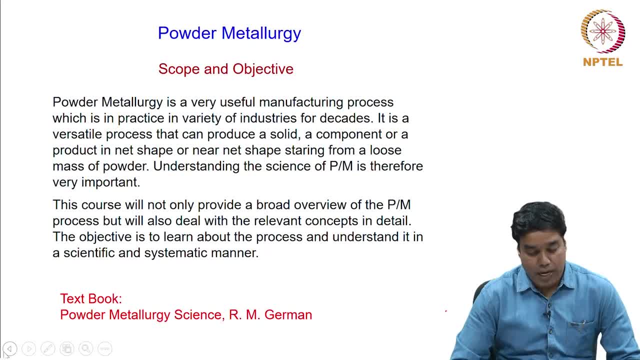 starting from a loose mass of powder, and therefore understanding the science of powder metallurgy is very important. This particular course will not only provide a broad overview of the powder metallurgy process, but we will also deal with the relevant concepts in detail. The objective is to learn about the process and understand it in 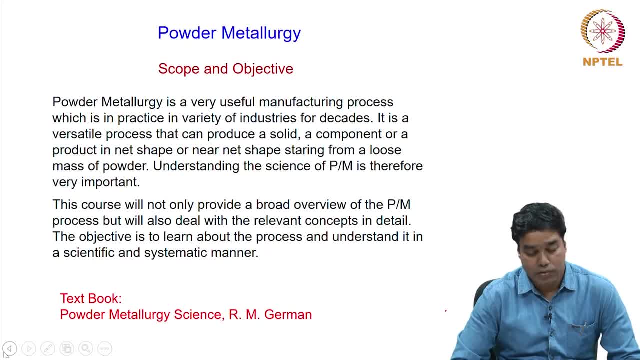 a scientific and systematic manner. ok, So in a nutshell, the main objective of this particular course is to learn in great detail about the entire process of powder metallurgy, as to how it is done, what are the relevant mechanisms and concepts and all other details. 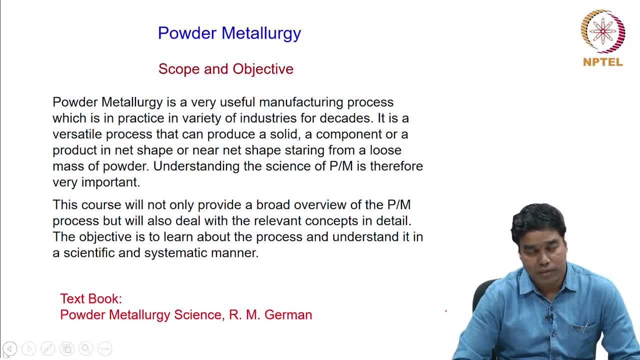 associated with this particular manufacturing process called powder metallurgy. ok, The book that you can refer to for this particular course is a book by R M German. In fact, this book is known as the Bible of Powder Metallurgy. The book goes by the same name. 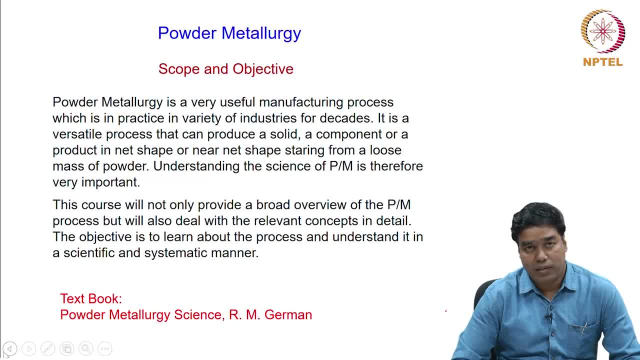 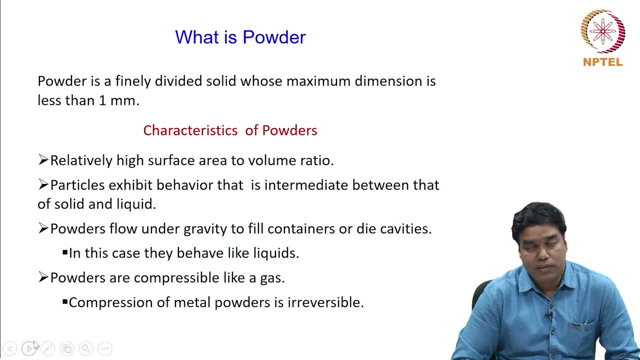 Powder Metallurgy Science, and the author is R M German, So you can refer to this particular book for most of the things which will be covered in this particular course. ok, Let me tell you what is a powder, because that is what we start with in a powder metallurgy. 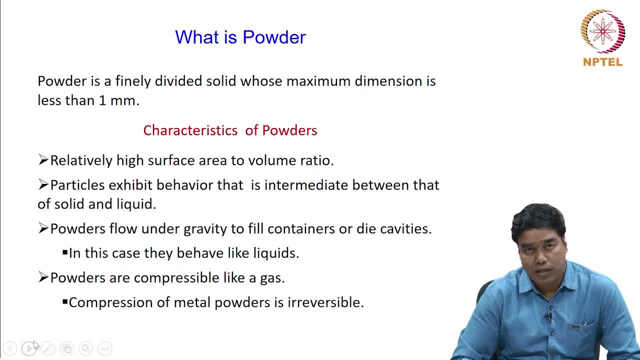 I suppose you have already gone through the syllabus and you have seen what are the topics which will be covered in this particular course and the different categories or subtopics which are there under English, Each of these topics. So the first thing that you start with in a powder metallurgy process is 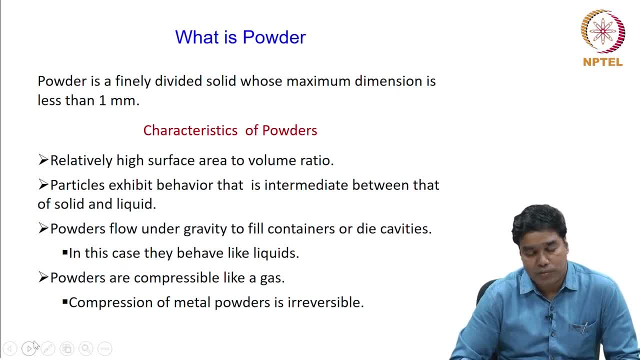 the powder itself, as I was mentioning. So first you need to know, or you need to understand, what is a powder, right? So powder, if you want to define as such a powder can be defined as a fine, finely divided solid whose maximum dimension is less than 1 millimeter. ok, So in a broad 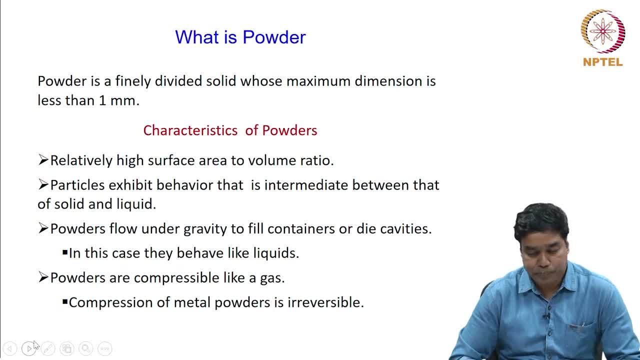 term. that is how you can define a powder, but a powder also should have a certain characteristics, which are listed over here, as you could see, and the characteristics that a powder should have are as follows: It should have a relatively high surface area to volume ratio. The powder particles exhibit. 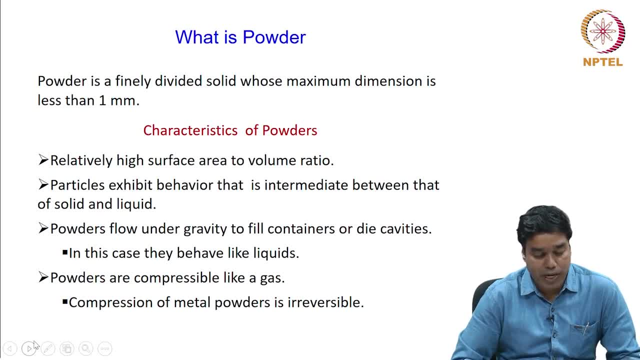 behavior that is intermediate between that of solid and liquid. For example, powders flow under gravity to fill containers or die cavities and in this case they behave like liquids because they are flowing and they can go To you know, different places inside a mold, for example when you are molding the powder. So 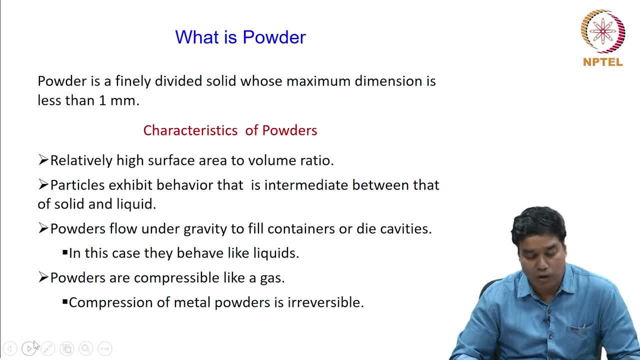 like how a liquid flow, the powder particles can also flow and that is why it is said that you know their characteristics is in between that of solid and liquid. ok, Powders are compressible like a gas, and compression of a metal powder is irreversible. That means 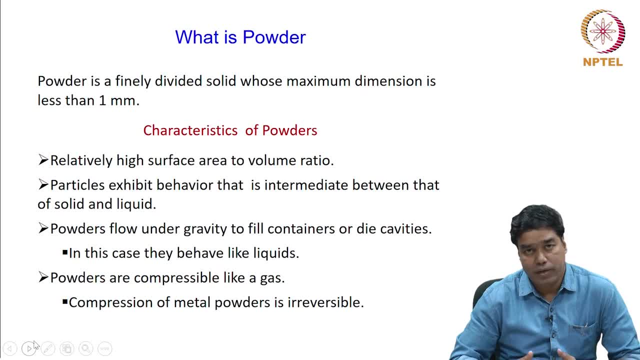 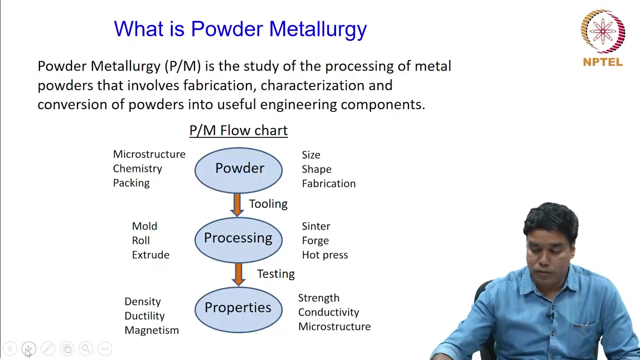 once you compress it or compact it, you cannot get it back to the initial condition. So these are the typical characteristics that a powder should have, apart from the fact that the dimension of powder particles, or the solid which can be called a powder, should be less than 1 millimeter. So that is about the powder. Now, when you 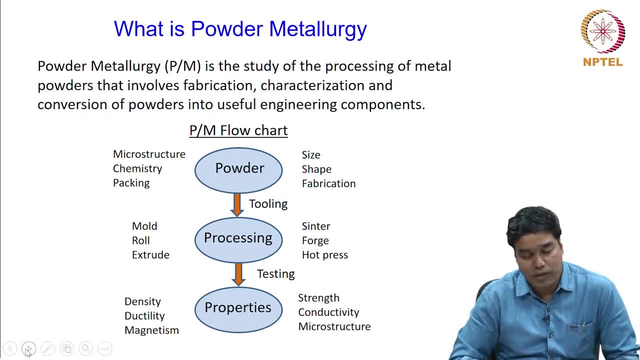 say powder metallurgy. as I said in the beginning during the introduction, powder metallurgy is a whole manufacturing process which can be used to make products and components. So powder metallurgy, if you want to define it, can be defined as the study of the processing of metal powders. that involves fabrication, characterization. 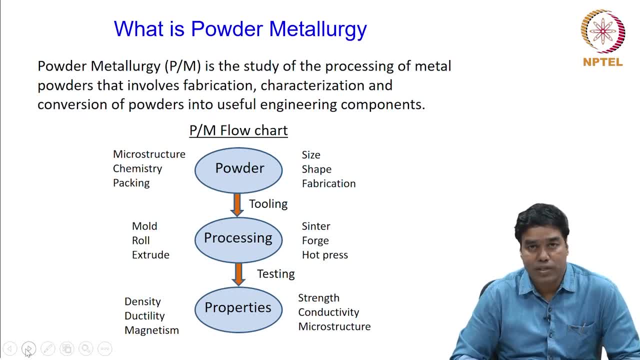 and conversion of powders into useful engineering components. right, So you start with the powder and then you can make components or you end up with a final product. right, So that means the powder has to go through certain steps or certain processing in order for you to get a 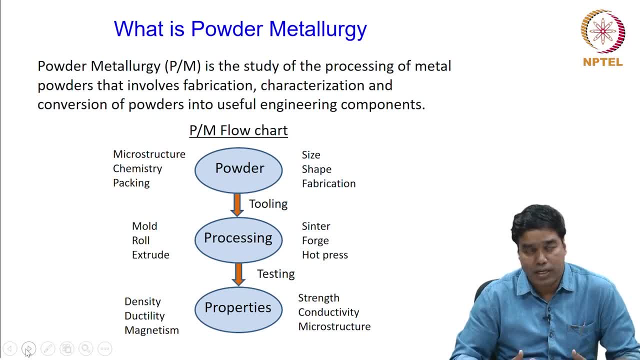 useful component or a useful product at the end of the process. ok, So that is how you can see. it is listed in the powder metallurgy flow chart, as you could see over here. As I said, you first start with the powder and you have to process the powder to get a particular component. 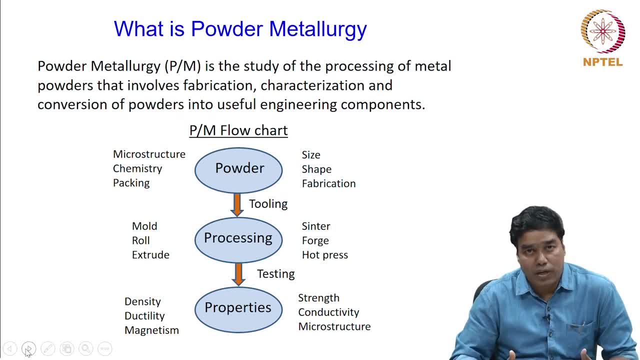 or a particular product with required properties. So when you process the powder you need certain toolings which can process it and, you know, give it a particular shape and things like that. And after that, once you process the powder into a solid, you need to test its properties so that you know that whatever desired properties, 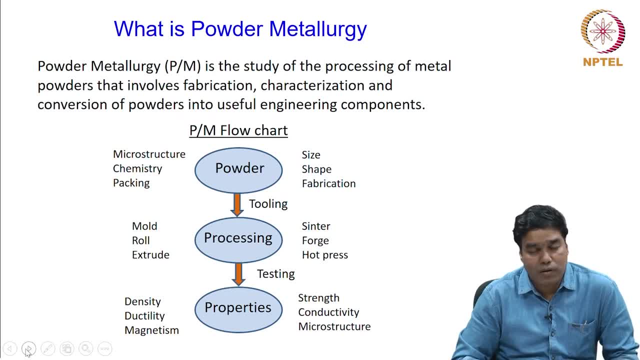 which you wanted in a, in a particular component or in a particular product, is there in the, in the final part or in the final product which is coming out at the end of the powder metallurgy process, right? So when you check these properties, you need to do some testing also. So 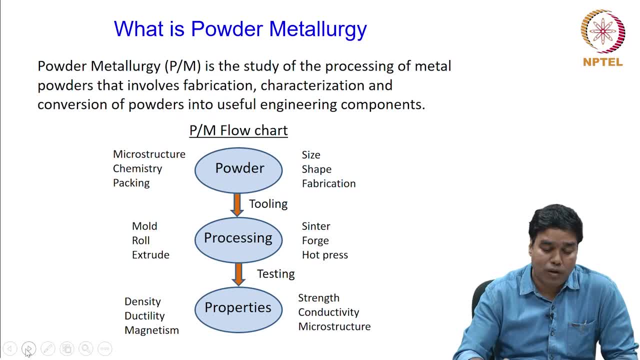 that is how you can see how the flow chart goes over here: powder, then with the tooling you process the powder and then you want to get certain properties. So you need to test it to get to know whether those properties are achieved. ok, 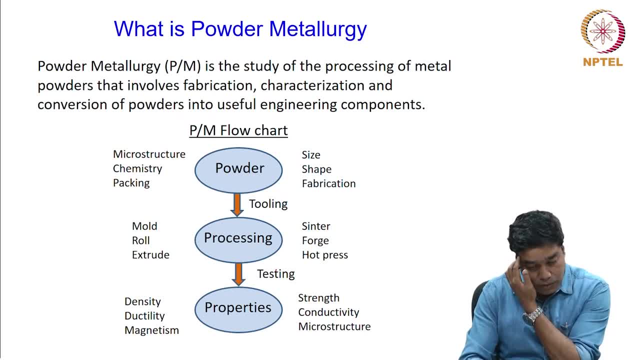 So now, in each of these steps, you have certain parameters that you need to consider, certain factors that you need to consider, For example, when you talk about the powder itself. the powder has certain properties or certain characteristics in terms of the size, the 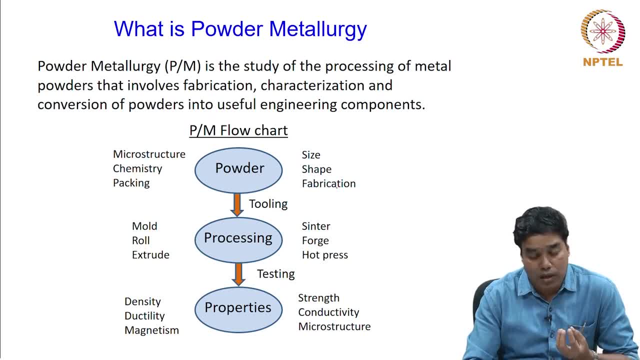 shape and the fabrication process that is being used to make these powders, And, apart from that, the powder also have certain properties, like the microstructure, the chemistry of the powder and also the packing, because all these parameters will decide how the processing would be. 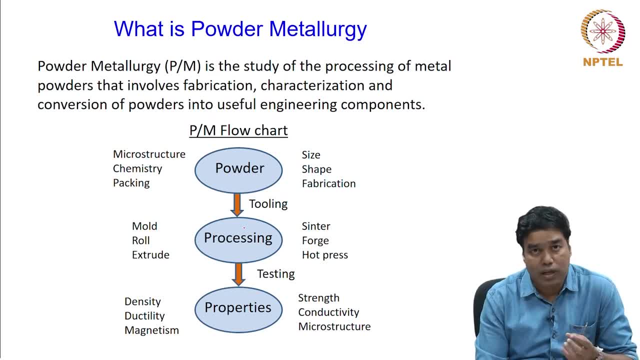 Because the powder has to be packed first in a particular shape. right? So how that packing would be, that might depend on one or more of these parameters which are listed over here, like size, shape or microstructure, chemistry, packing and so on. right? So before 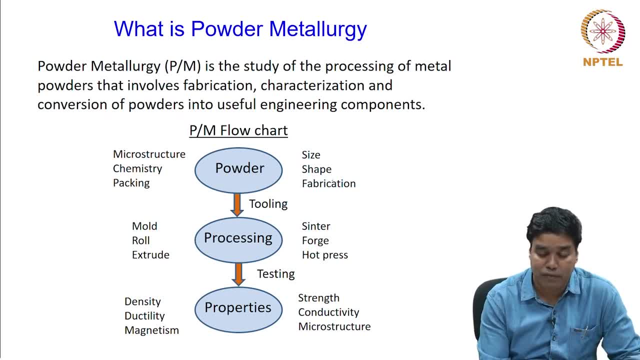 you actually start the processing. these factors or these parameters have to be evaluated So that you know you are dealing with what kind of powder and what it might lead to when you process the powder for making a particular component or product. ok, Now in the next step, while you process the powder- as I said before also you need certain 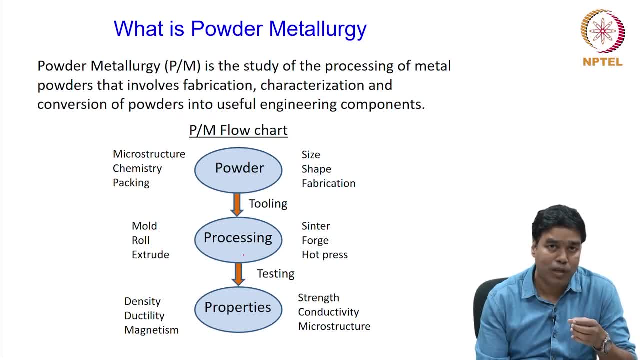 tools. For example, you have to mold the powder in a die and then it has to be compressed Right. So in order to do that, you need that die, the punches which will compress it, and also a press which can apply the pressure on this loose powder and give rise to a compact. 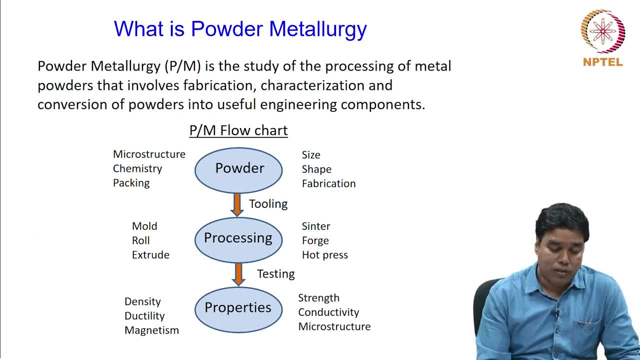 which can be further processed. right? So here the parameters could be like the mold when you do the molding, or or the process, or the toolings, if you talk about it, will it? it can be molding, rolling or extrusion of the powder in order to give it a particular 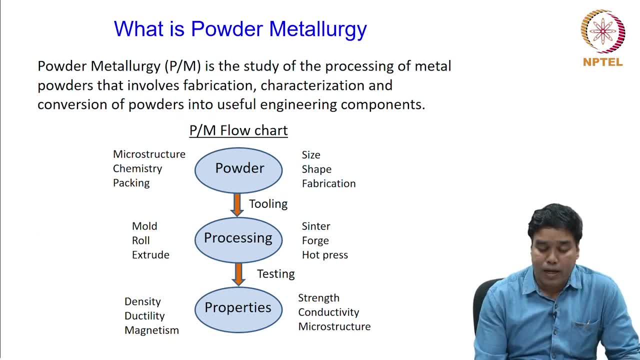 kind of shape and compact it And, on the other hand, once you have the compact, after either molding, rolling or extrusion, you need to finally close all the pores which are there in this compact Right. So you need to close all the pores which are there in. 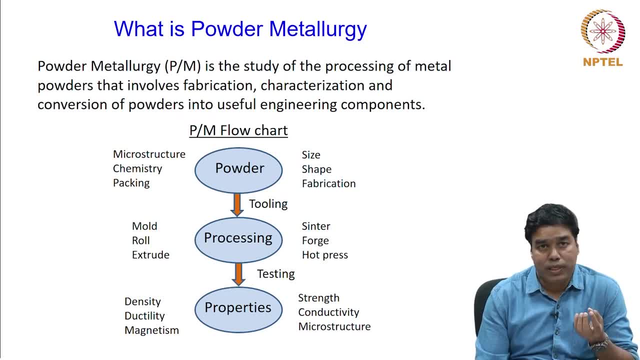 this compact So that at the end, you come up with a fully dense, solid right. So that is the, the final product that you need. the final product should be fully dense And in order to achieve that, you need to either sinter the powder, forge it or hot press it. So 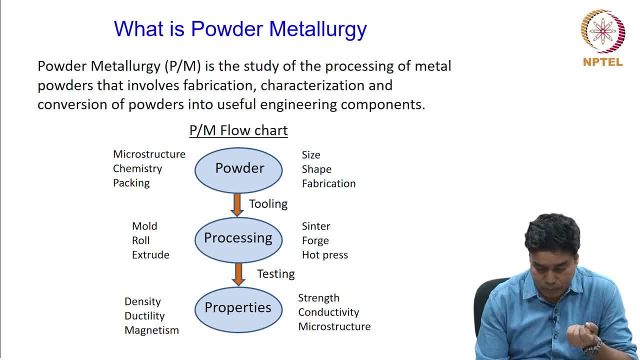 these are all high temperature process sintering, forging or hot pressing, which will make sure that whatever the temperature of the powder is, So that is the final product that you will get. So you need to take whatever porosity is remaining after molding, rolling or extrusion. 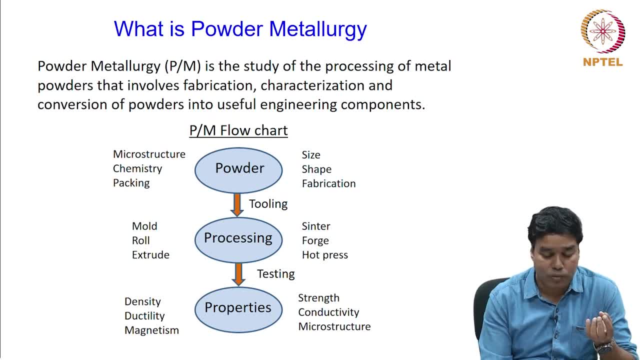 after the compact is made through one of these processes: The sintering, forging and hot pressing. this high temperature processes will make sure that the pores are closed and at the end, you get a fully dense product. ok, So this is how the powder will be processed, with the help of certain tools and certain 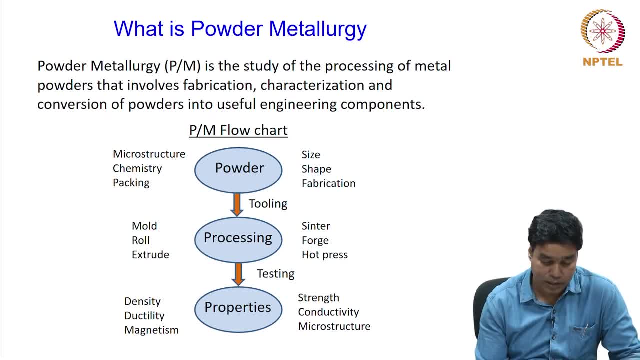 processes like sintering, forging or hot pressing, which happens at the high temperature. Now, finally, once you you make a solid part out of it, you also look for certain properties, which could be any of these. For example, you look for strength, you look for conductivity, or 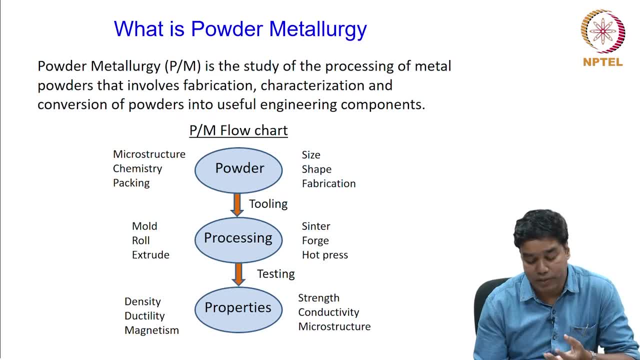 you look for a particular type of microstructure which can again give rise to certain type of property that you need in that particular component, And the other properties that you may look for is the density. as I said, at the end you have to have a product or a component coming. 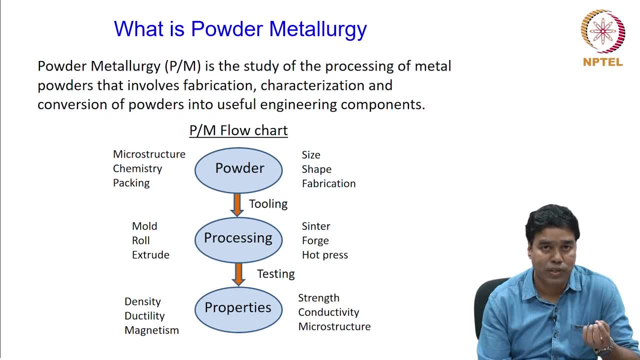 out from the process, which should be fully dense. So you need to evaluate and measure the density And then, when you talk about mechanical properties, you also have to see what is the ductility of the final product and other properties like, for example, magnetism, right? So, depending on what your requirement is or what the 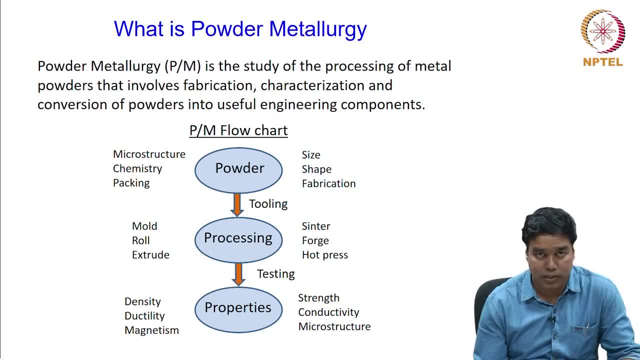 properties that you are looking at. you do the testing and evaluate those properties right. So if I have to summarize now the powder metallurgy process, it starts with the powder. the powder is processed In the compact or into a particular shape, which could be the near net shape also. 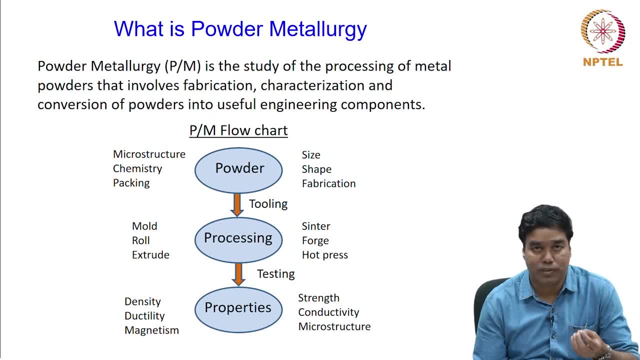 And then it is densified with the help of a high temperature process like sintering, forging or hot pressing, And then, once you obtain a final, fully dense product, you evaluate the properties depending on what are the requirements or what are the properties that you are looking. 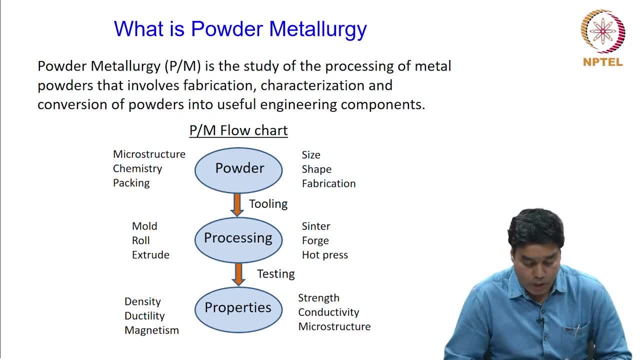 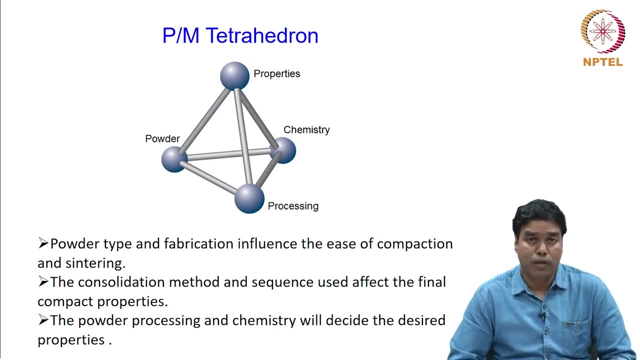 at ok. So how this processing and properties are interrelated or correlated, that can be understood with the help of a diagram like this, with the help of this tetrahedron, which is known as the powder metallurgic tetrahedron, where you can see in each of these vertices you have this 4. 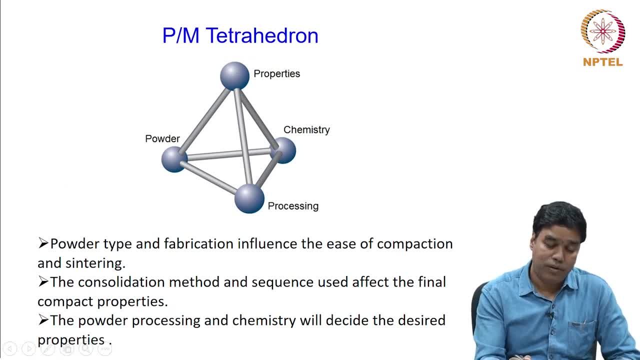 different parameters or 4 different things listed. ok, The powder, that is, the starting material, as I said. the processing, the chemistry and the properties. ok, So the way this powder, metallurgic tetrahedron can be used to process the material. So the way this powder. 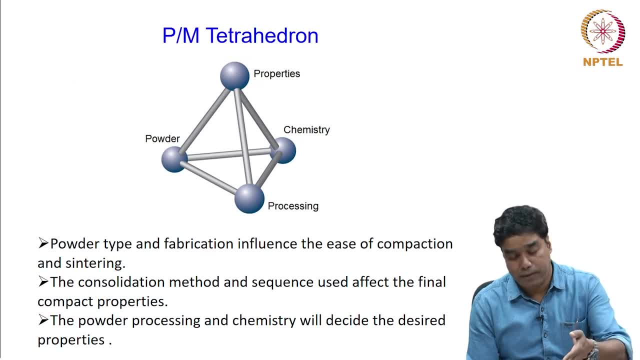 metallurgic tetrahedron can be used to process the material. So the way this things are correlated, you can easily see it from this one diagram. For example, the powder is related to how it can be processed ok, or how easily it will be processed, or whether 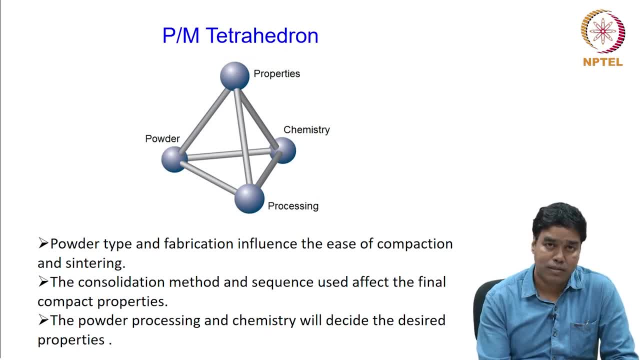 it will be difficult to process. that would depend on the characteristics of the powder, So, for example, the powder type and the fabrication that can influence the ease of compaction and sintering, Because what you do while making anything out of a powder, 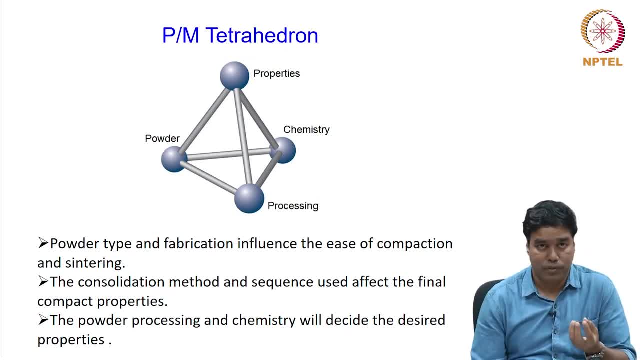 you first compact the powder into a particular shape. So you try and give give it a shape in the beginning by compacting it, and then you sinter that compact to close all the pores and come up with a fully dense product. ok, So how the powder? 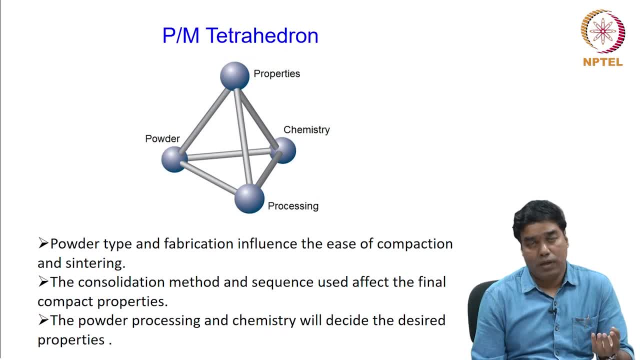 is in the beginning, in terms of its type or the fabrication process which is used to to make the powder, that will influence the ease of compaction and sintering. ok, So that is how these two, this powder and processing- this is how you know these two things are related to each other. 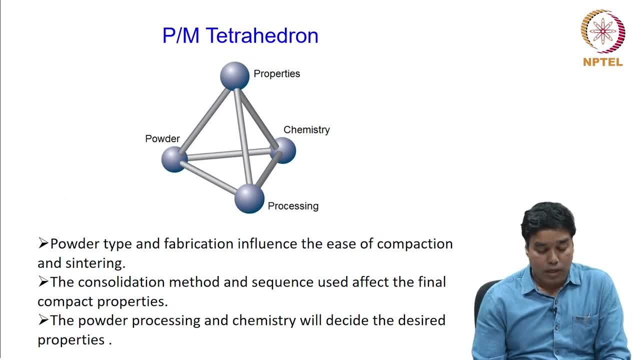 Similarly, how the powder is processed will influence the final product. So this is how the final properties ok, And in between you have chemistry, because chemistry also has a lot to do with the processing and also the properties. If you change the chemistry of the material, 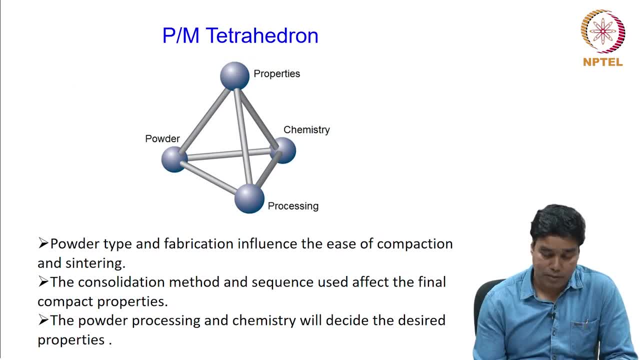 that will also change the properties, right. So this is how these vertices are correlated to each other. This is what we also call as a structure property correlation, where you have the final properties ok, And in between you have the final properties ok, And. 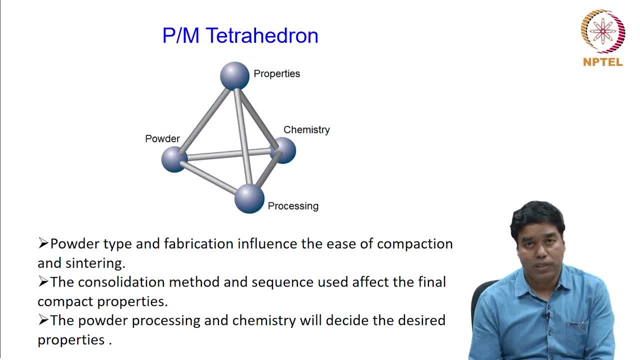 you, you make something, you process something which will give rise to a particular chemistry or a particular structure, And the properties that you obtain. finally, that would depend on the structure right. On the other hand, how the material is processed, the structure would depend. 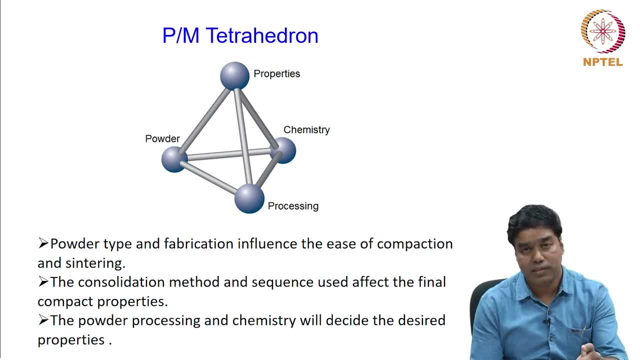 on that. And processing, as I said, in this case of powder metallurgy, in this particular case, processing would depend on what kind of powder you start with, right. So this is how, with the help of this powder metallurgy tetrahedron, you can see how these four things are correlated with each other. ok, Now when. 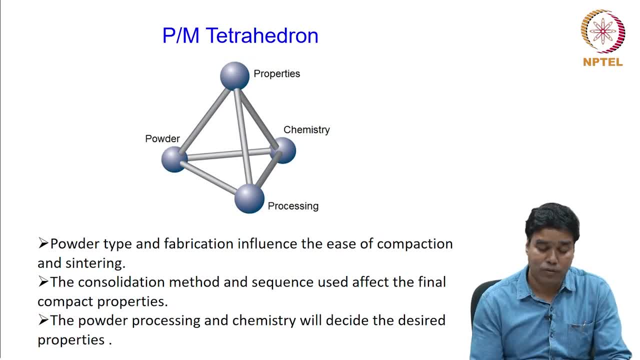 you look for the properties or you want to know the chemistry, you will have to actually test it right. You have to measure it. Then only you have to measure it. Then only you can know a particular property, whether it is achieved or not, in that particular compact or in. 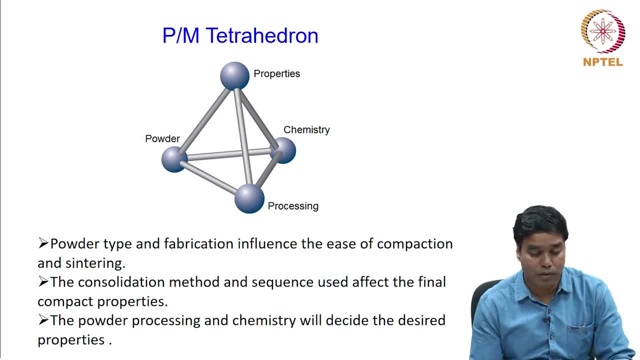 that particular component which is made out of the powder. ok, So in order to know that, you know, you need to actually characterize the material which has been processed right. So that is why characterization is at the center of this tetrahedron, because for each of these that you 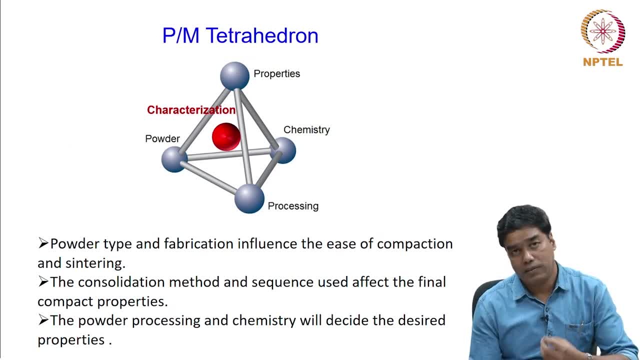 you want to know whether it is the chemistry or it is any particular property, you need to actually test it and in order to test it, you need to characterize it. you need to measure that particular property using certain tools, right? So that is why you also need to bring 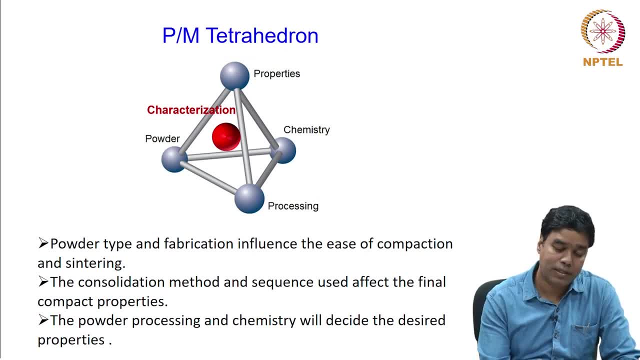 in the, the process of characterization here which is at the center, because for each of this, as I said, you need to characterize. For example, if you need to know what kind of powder, it is, the type of powder, then you need to actually see the powder under a microscope and look at the. 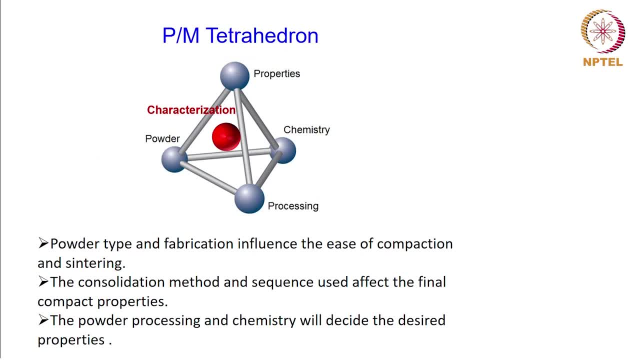 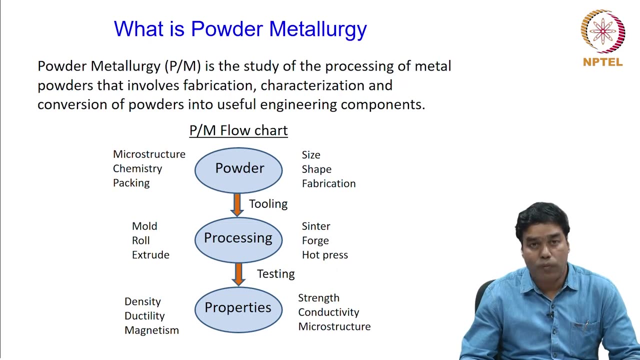 powder particles. So that is a characterization tool in that case, which you used to get to know about the powdありがとうございました on it right. using a particular instrument, One may ask a question as to why powder metallurgy and why not any other process. 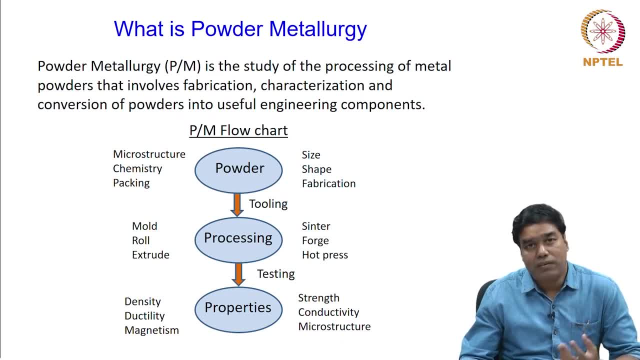 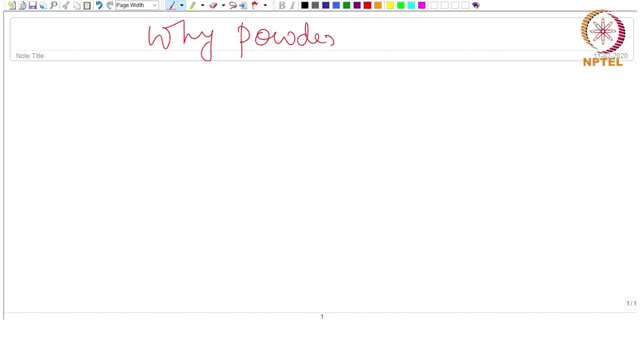 or Any other methods. In other words, what is the advantage ofpowder metallurgy over many other manufacturing processes which are available? ok, So let us try and understand as towhy powder metallurgy and what will be the advantage of powder metallurgy overmany othermanufacturing processes. ok, 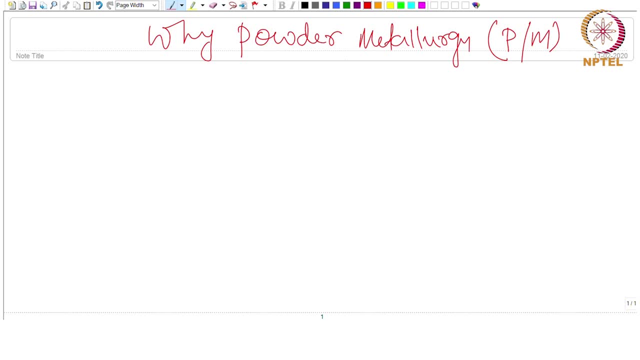 Why powder metallurgy? This can be understoodwith the simple vein Vein diagram, which will show up the capability of a particular process and, as far as the powder metallurgy process is concerned, with the help of this diagram, we are going to see what are thosecapabilities that powder metallurgy process will offer, and how it is different. 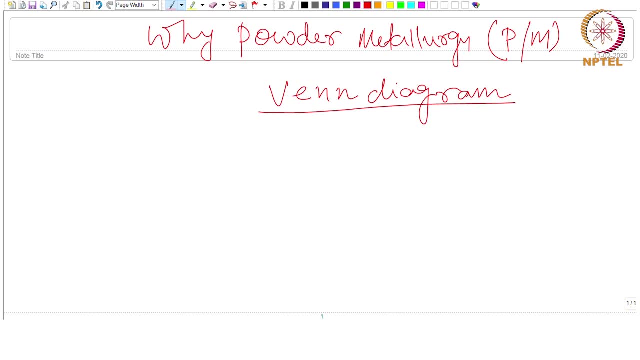 or how it is advantages This compared to other processes? So this is how a vein diagram looks like, and each of these circles can be associated with a particular property or a particular capability. Let us say, for example, this first circle that you have. 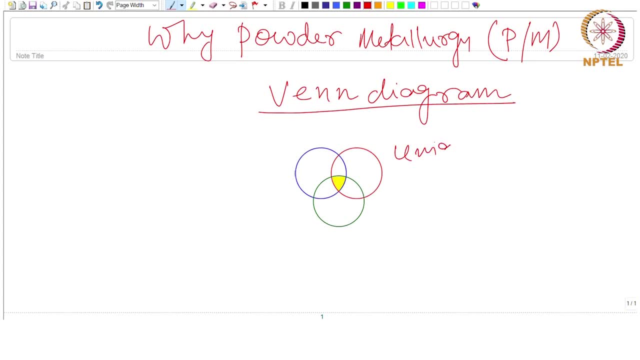 It see, that is talks about the uniqueness of the process, which can be in terms ofthe material, like the alloys, or a particular type of microstructure that one wants to produce. Now, it is in detail. I am not adding details about that. 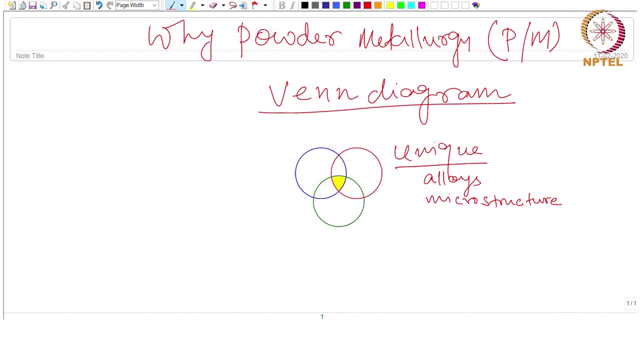 in a particular alloy or in a particular material and a particular type of material that somebody wants. let us say, for example, you want composites which are combination of two or more materials. ok, So that can be done with this process of powder metallurgy. we can also make certain alloys that. 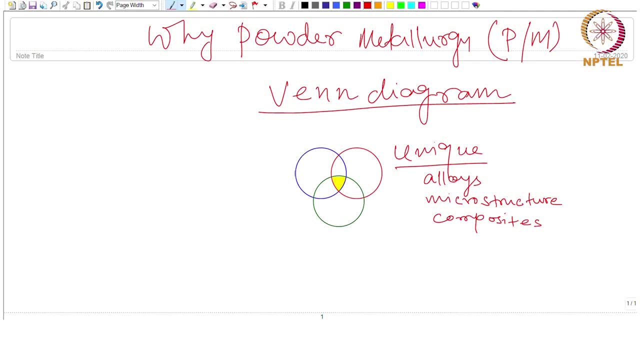 means you can have different chemistry and come up with, you know, different kinds of alloys. You can also tailor the microstructure and so on. So that is the uniqueness of the process. And then, when you talk about any manufacturing process, the other aspects that you will have to consider is, of course, the economy. 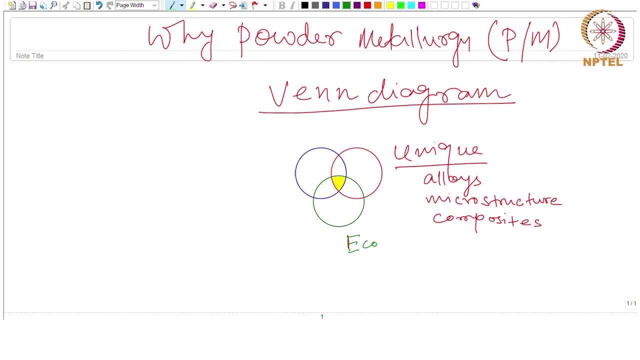 Because when you are comparing this process with any other manufacturing process, you also have to look at the cost: whether it is cost effective or not compared to many other processes. So when you talk about cost, you should also look at the precision and the productivity, because 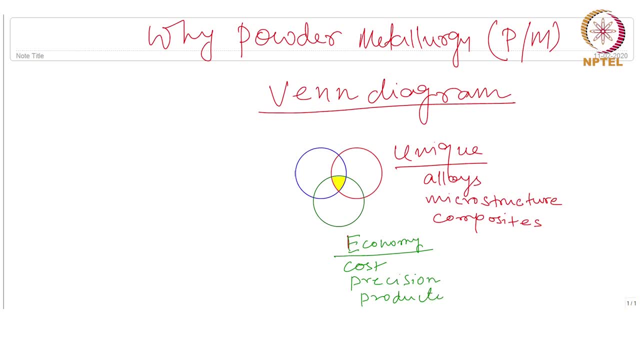 these two are also related to the total cost of the process. For example, the rate of production or the productivity would of course lead to you know how higher or lower cost, depending on whether you have high productivity or low productivity. right, And then the third. 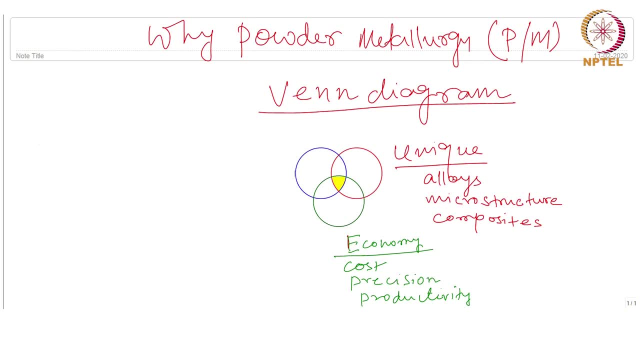 circle can be assigned to another capability of the process, Which is captive. that means this process is capable of processing materials which are difficult to process by other conventional processing or manufacturing routes. For example, this refractory or reactive metals, or refractory or fracture metal. So this, where the material is more scroll, like tungsten, which is 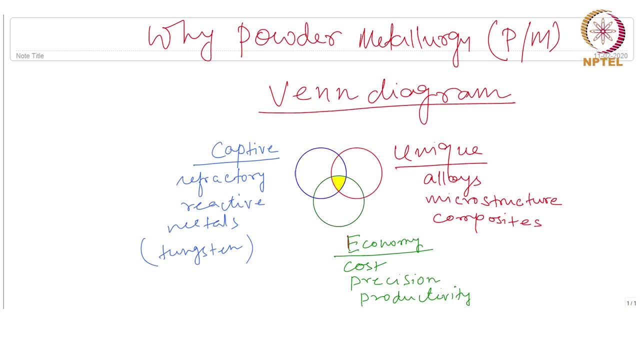 a refractory metal. Refractory metal means the melting point is very high so it is difficult to melt. So let us say you want to use a conventional manufacturing route like casting, then you will find it difficult to melt because in casting process you have 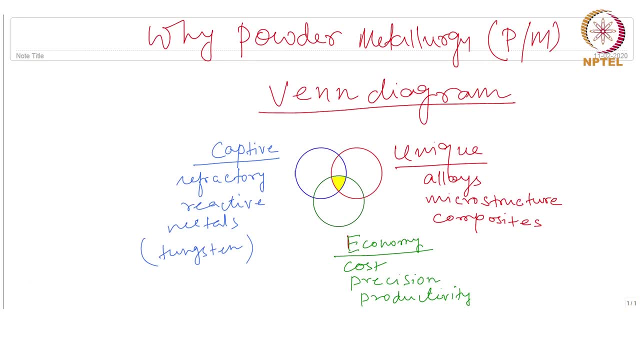 to first melt the material and then cast it and solidify it. So, since it is a refractory metal, if you want to use a conventional processing or manufacturing route like casting, it is going to be difficult, but powder metallurgy can easily handle that, you know, and overcome the difficulties. 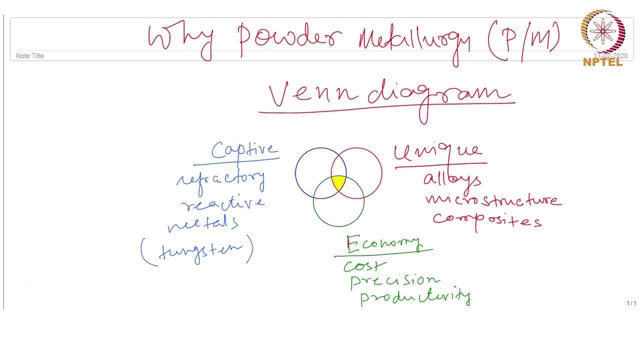 that you might face while using a conventional manufacturing process. Similarly, if you have a reacting, reactive metals, for example, titanium, zirconium and this kind of metals which are prone to oxidation if you process them at high temperature, Any way, you will have to process. 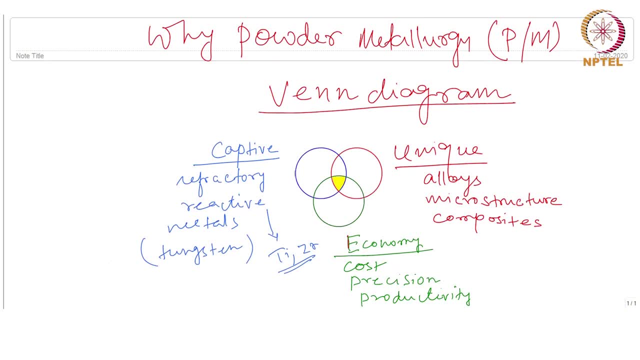 it at high temperature, right? So this kind of metals are prone to oxidation or other reactions and that is why this kind of reactive metals are difficult to process by hand. So if you are using a conventional manufacturing production process like casting, conventional processing routes, but powder metallurgy can easily take care of that, ok, 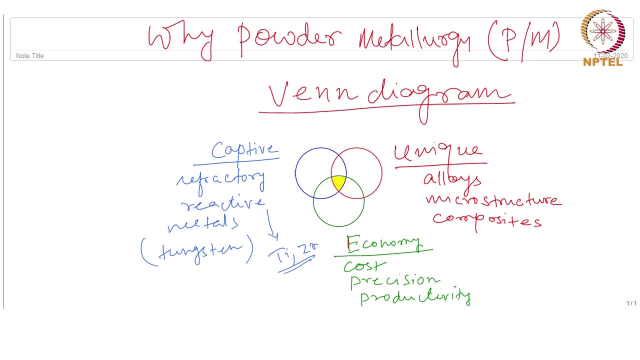 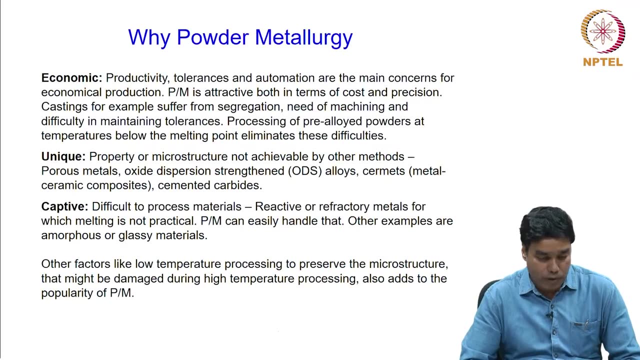 So, if I can elaborate on this, these are those 3 capabilities of this powder metallurgy process, starting from the economy, which also concerns the productivity, the tolerances and automations. So powder metallurgy is attractive both in terms of the cost and the precision. 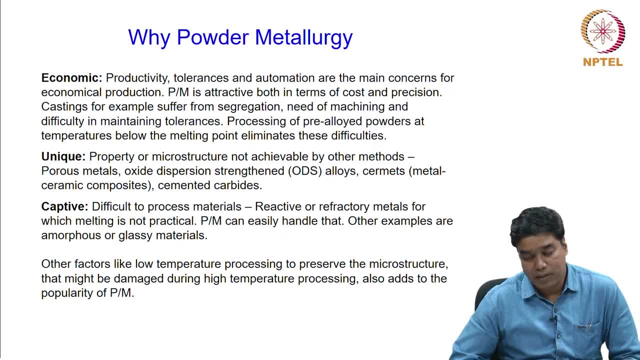 because, as I said in the beginning, it can also make the product in net shape or near net shape. So your requirements for machining and things like that is much lower. So it is. it can easily make a product with high precision. Other manufacturing processes, for example. 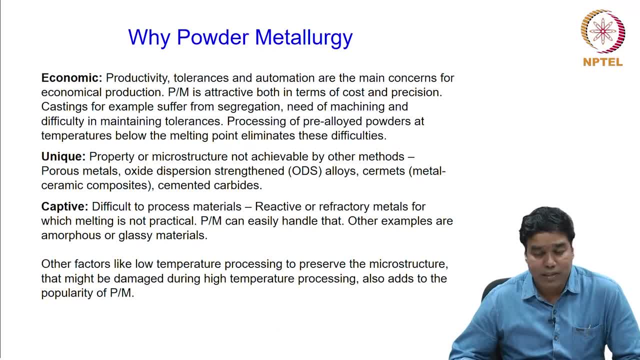 castings suffer from defects like segregation, and there is also need for machining, and it is difficult to maintain the tolerances right. So these kind of difficulties are not there in case of powder metallurgy, and that is why this is attractive in terms of both economy. 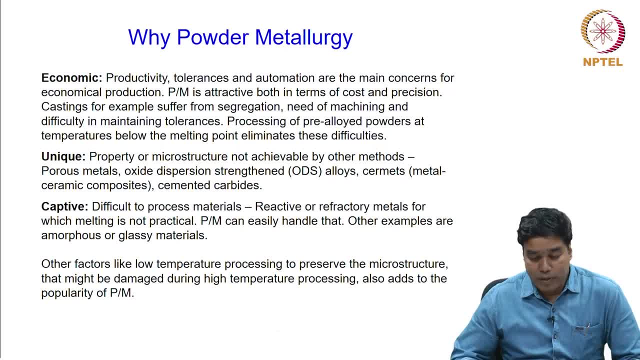 productivity and the tolerances. Moreover, processing of pre-alloyed powders at temperature below the melting point also eliminates many of these difficulties which are associated with high temperature processing. like you know, this segregation, porosity and so on. Then, if you talk about the uniqueness, this will come in terms of a property that you are. 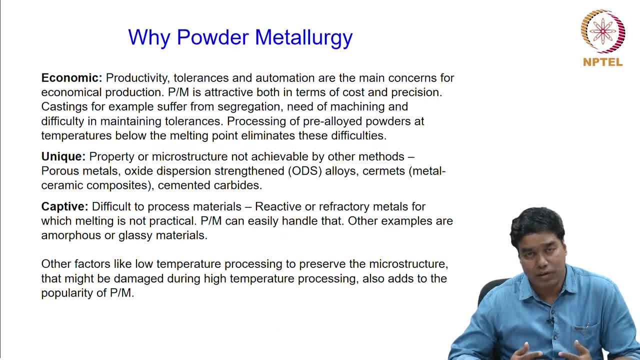 looking for, or a particular type of microstructure that you are. you are looking for in the material for a particular type of property which will come out from that, that kind of microstructure, right. So property or microstructure which cannot be achieved by other methods can easily. 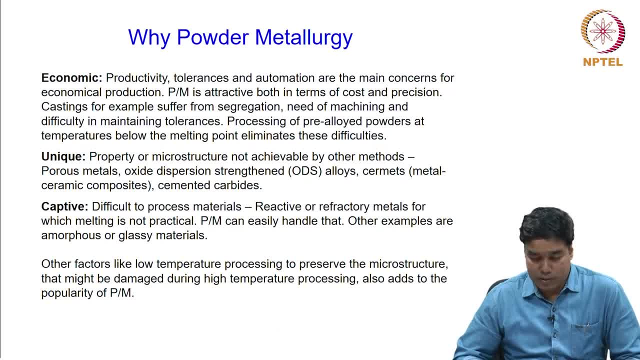 be obtained by a powder metallurgy process. ok, For example, porous metals, oxide dispersion strengthen alloys which are much stronger Then cermets, which is a combination of ceramic and metal. that is how the name is, cermet it is. it is a combination of ceramic and metals. So 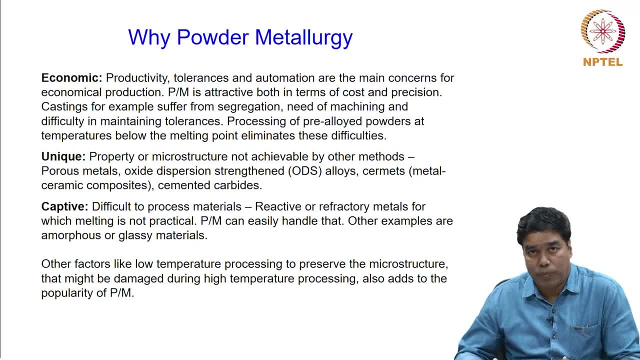 you also achieve a combination of properties, that of ceramics and metals in a, in a single material, when you combine them as a cermet right. So this kind of cermet materials can also be processed with the with the help of powder metallurgy. 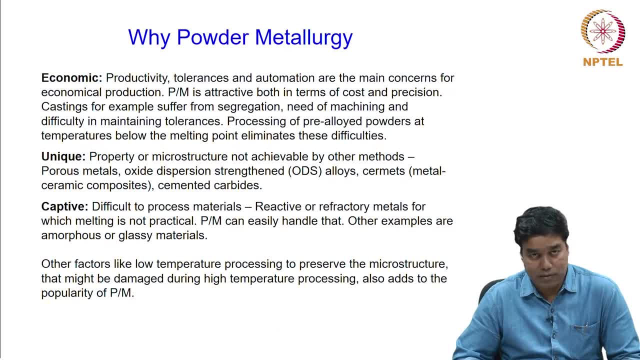 And other specialty materials, for example cemented carbides, which are again difficult to process by conventional processing routes, can also be processed easily by powder metallurgy. So that is how the process is unique, And when you talk about the captive characteristic of this particular process, it it talks about the difficult to process. 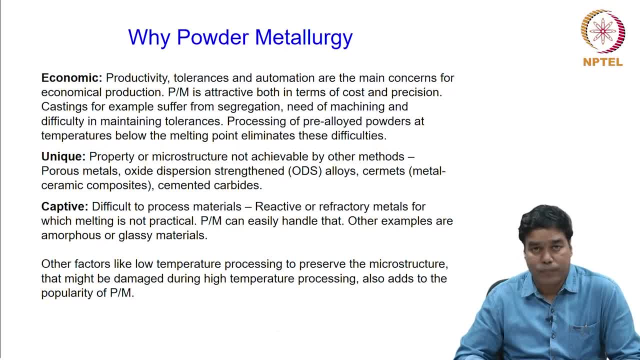 materials, or the ability of this process of powder metallurgy to handle the materials which which are difficult to process by other processing routes, For example, reactive or refactor metals, as we talked about, which are difficult to melt. ok, And since you know, they are highly reactive and melting temperatures are very high. 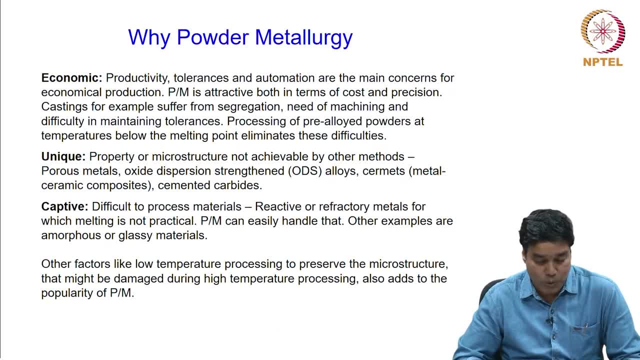 it is also not practical to go for melting and casting route. but powder metallurgy can easily handle that, because here you do it in in solid state itself and there is no need for melting to to process this kind of cermet. So it is very easy to process this kind of cermet. So you can 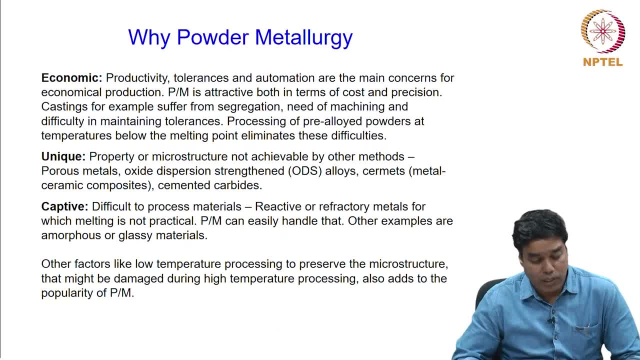 use those kinds of materials. Moreover, you can also get a a kind of material which may be again difficult to process by other routes, For example this amorphous or glassy materials which are not crystalline, because what happens in other processes, like for example casting, when you 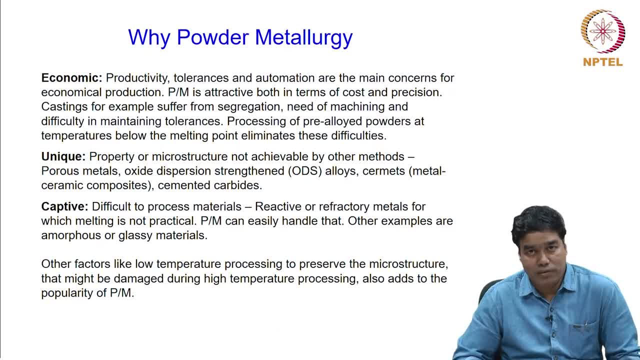 cool the material to solidify under equilibrium conditions, which is most often the case during the distillation. So when you are adding the mate, when you are adding the discharges or the salt adhesion process, that is what is going to happen, But then you can also get a kind of 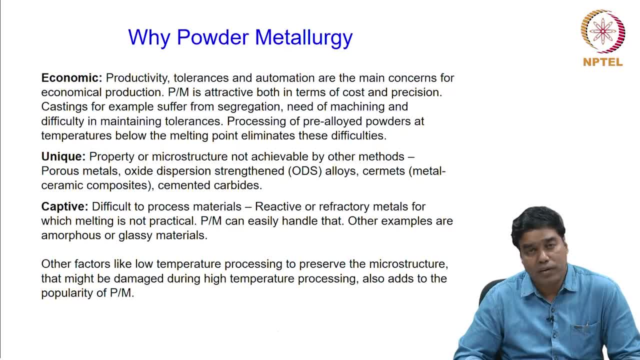 materials which may be again difficult to process by other routes, For example these amorphous or glassy, a particular process. When you cool it under equilibrium conditions, it most of the time it will- it will solidify into a crystalline material. So for some reason, if you want an, 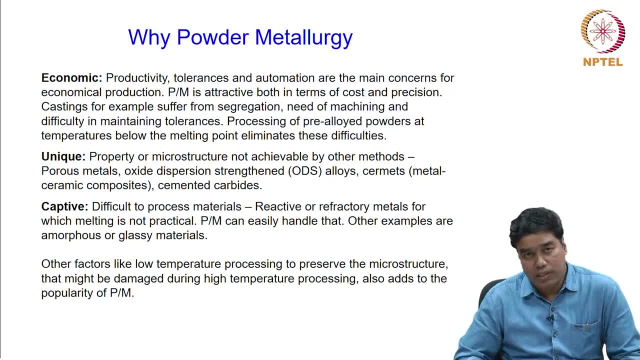 amorphous or a glassy material as we call them, then it will be difficult to use those kind of processes. But powder metallurgy, if you take care of some of the process parameters, can also, you know, easily handle these kind of materials or easily produce these kind of materials. ok, 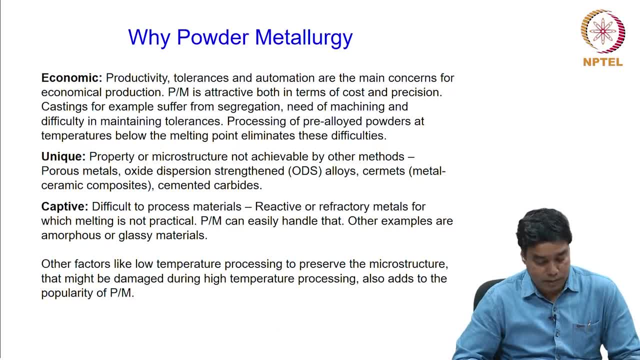 Then you have other factors, like low temperature processing to preserve a particular microstructure, because what happens when you process the material at higher temperatures? the microstructure that you wanted in the final product may be lost. For example, if you want a very fine grain microstructure, right, So that fine grain microstructure may be lost. if you 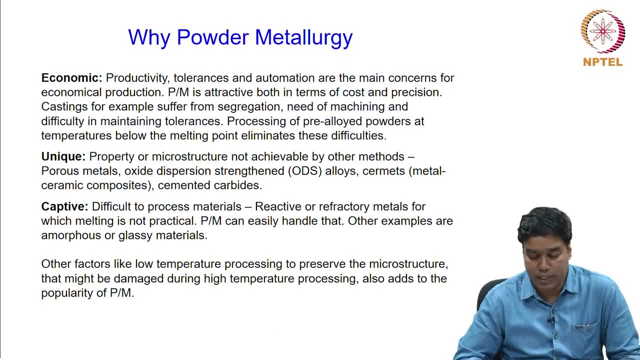 heat it to high temperatures because of grain growth, right, So that kind of requirements can also be taken care by low temperature processing. that powder metallurgy can do, And this again adds to the attractiveness or popularity of powder metallurgy. ok, So you know, these are the uniqueness or these are the characteristics of this powder metallurgy. 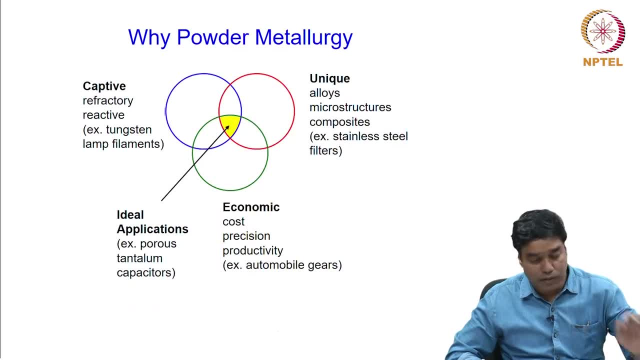 process, but the biggest advantage that you have in this process is what you can see in this junction, over here, right in this place, which is this, The meeting point of all these 3 circles, right, So in this place, you have all these 3 characteristics. 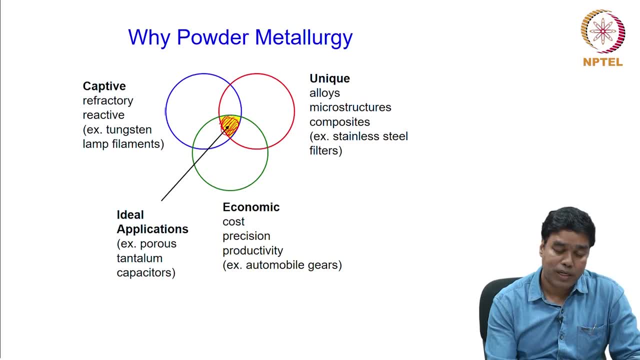 present. ok, So that means powder metallurgy can be an ideal application for making materials or making components products where you can combine all these characteristics in one process itself. So it could be ideal applications for specialty products, for example, like porous.